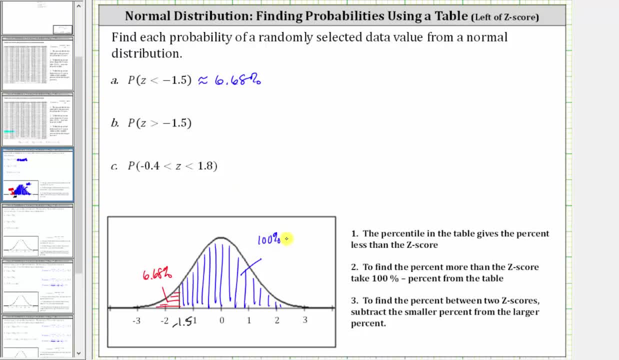 or the probability on the right. it would take 100% and then subtract 6.68%, which gives us 93.32%. So the probability the z-score is greater than negative 1.5 is approximately 93.32%. And then for the third example, 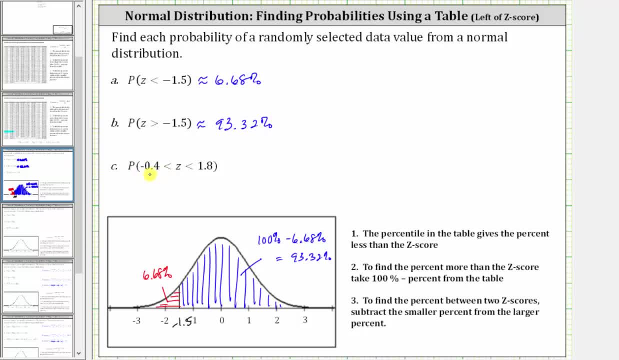 we're asked to find the probability that the z-score is greater than negative 0.4 and less than 1.8.. So let's go ahead and model this. on the standard normal distribution, The z-score of negative 0.4 is approximately here: 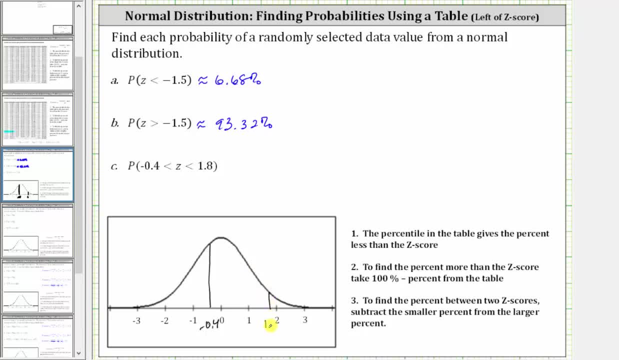 And the z-score of 1.8 is approximately here. So we're trying to find the probability the data value will have a z-score in this region here, To find the percent or probability between two z-scores, we subtract the smaller percent from the larger percent. 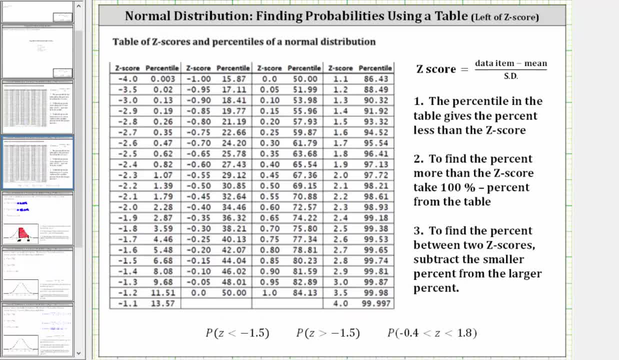 given in the table. So let's go back to our table and locate the z-scores of negative 0.4 and 1.8.. Negative 0.4 and negative 0.40 is here. The probability to the left is approximately 34.46%. 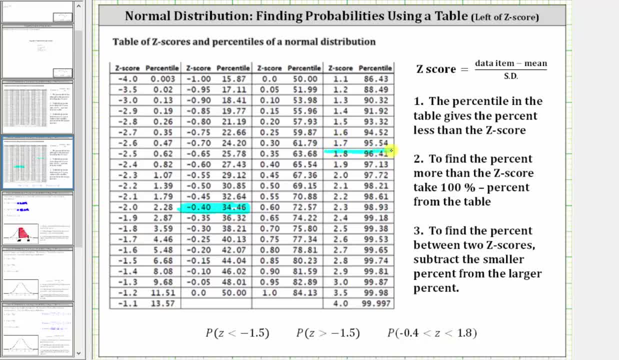 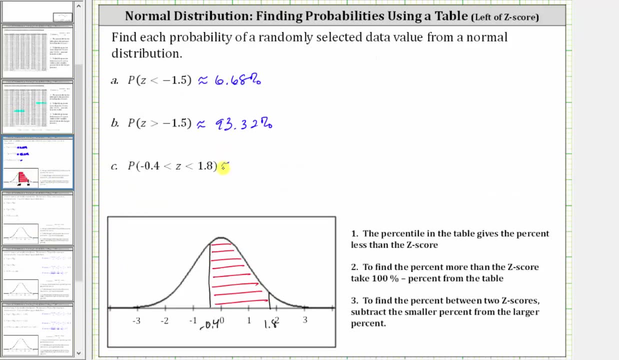 And the z-score of 1.8 is here. The probability to the left is approximately 96.41%. So to find the probability between the z-scores, we subtract 34.46% from 96.41%, So we have approximately 96.41% minus 34.46%. 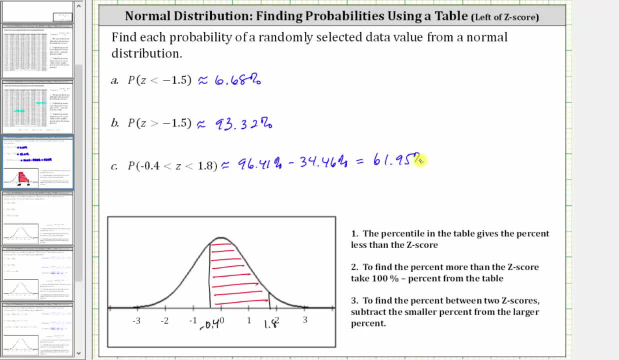 which is equal to 61.95%. And now let's look at our graph to see why we are subtracting these percentages. Remember, the percent or probabilities from the table give the probabilities of percent to the left. So if we subtract the probability, the z-score. 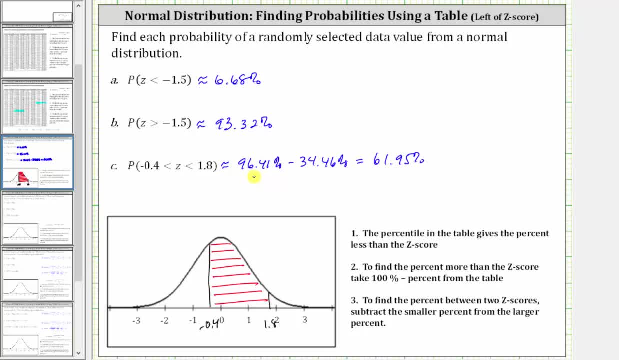 is in this region here. in this interval we took 96.41% and subtracted 34.46%, because the 96.41% gave us the probability to the left of 1.8.. Or the probability of the z-score is in this region here.